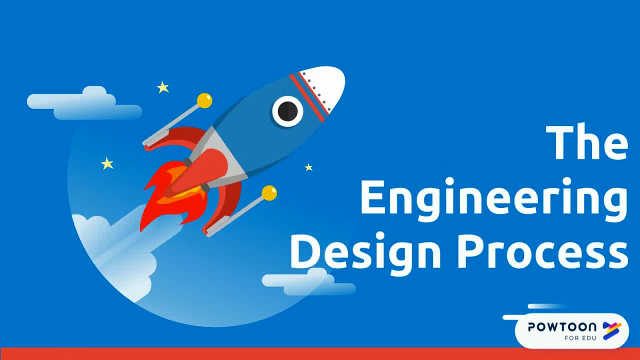 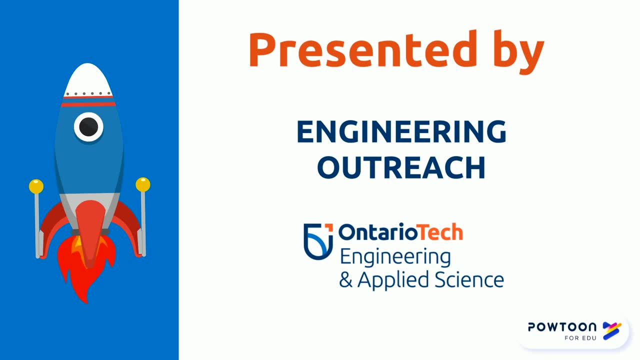 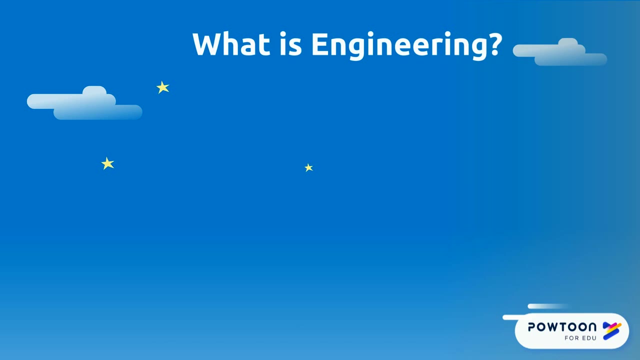 Today we're going to launch into the engineering design process and learn all about engineering, Proudly presented by Engineering Outreach at the Faculty of Engineering and Applied Science at Ontario Tech University. So what is engineering? Engineering is problem solving. Engineers look at the world around them and identify problems that they can solve with. 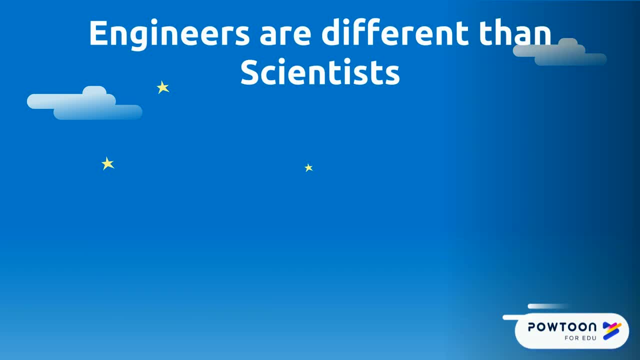 new ideas. Engineers are different than scientists. While both try to make the world a better place. scientists conduct experiments to better understand the world. Engineers, on the other hand, create designs to solve the world's problems, using skills like math, science and technology. 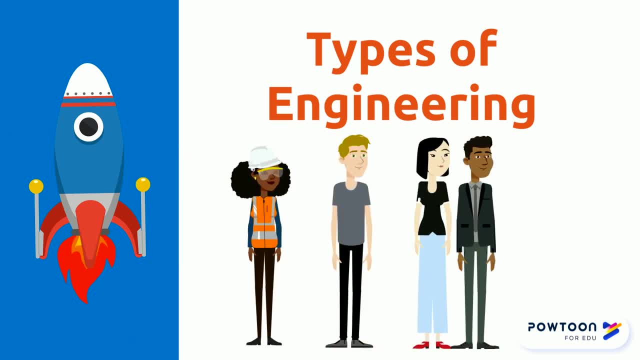 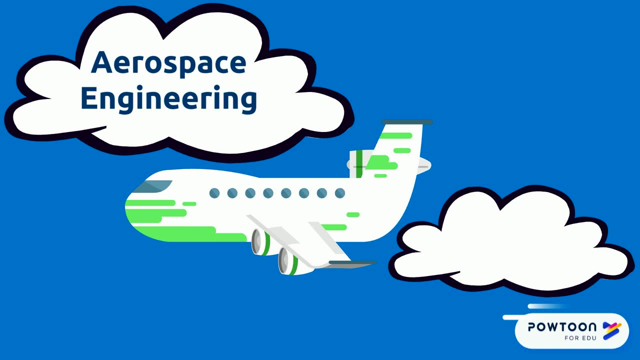 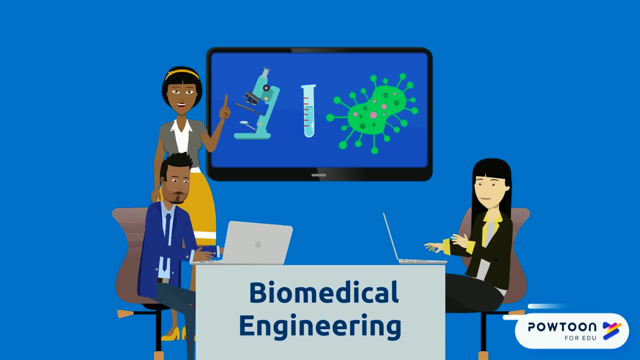 There are many different types of engineering. Different types of engineers solve different problems in the world. One type of engineering is aerospace engineering. This type of engineer deals with things that interact with the air, Things such as airplanes and rocket ships. Biomedical engineering solves problems within. 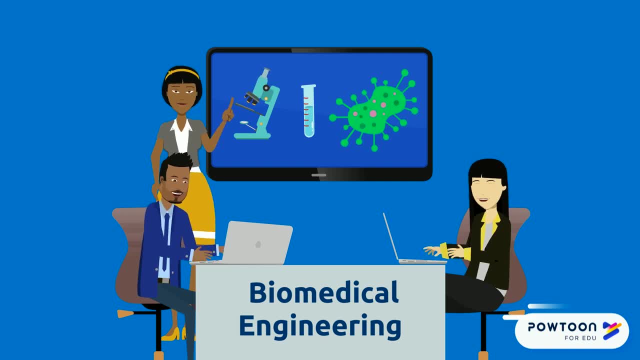 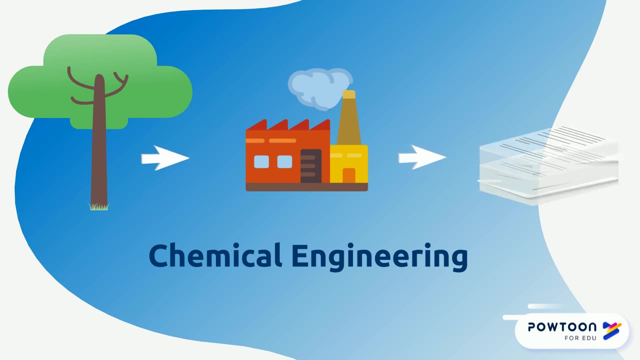 our health care system. Biomedical engineers can work on a bunch of different things, including creating things like prosthetics or helping with the diagnosis of disease. Chemical engineers are concerned about the process. They use all their knowledge to help find the most efficient way to create materials. for the most efficient way to create materials. 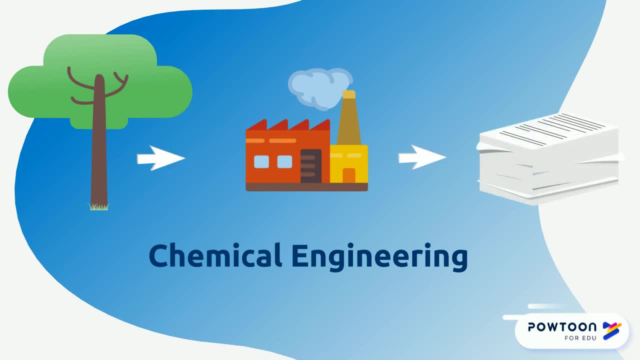 Chemical engineers are concerned about the process. They use all their knowledge to help find the most efficient way to create materials for the most efficient way to create materials or transform energy, such as in the process of making paper. Civil engineers deal with the design, construction and maintenance of structures. 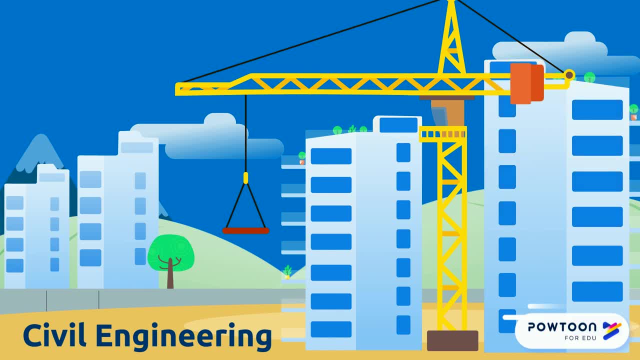 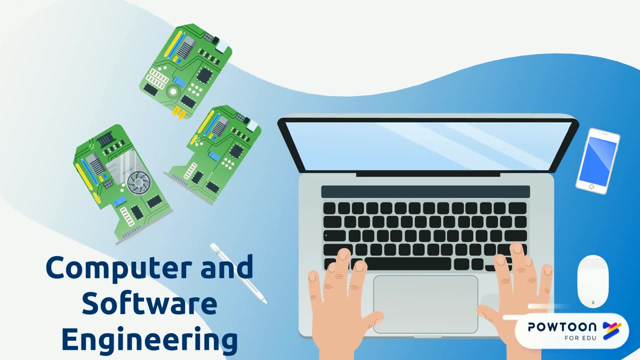 and infrastructures, Things like bridges, buildings and roads. The building you're sitting in right now probably has something to do with a civil engineer. Computer and software engineers deal with technology and help solve problems through the use of technology. They are responsible for coding and programming much of the things that we rely on. 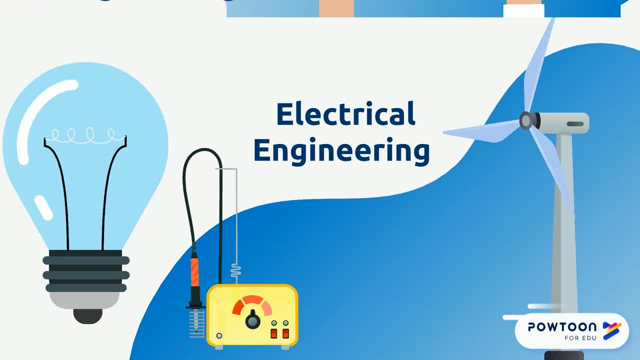 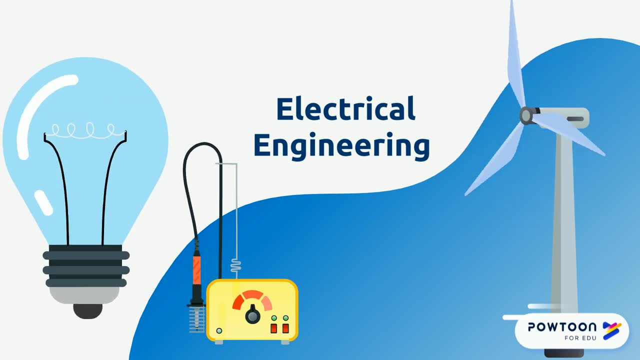 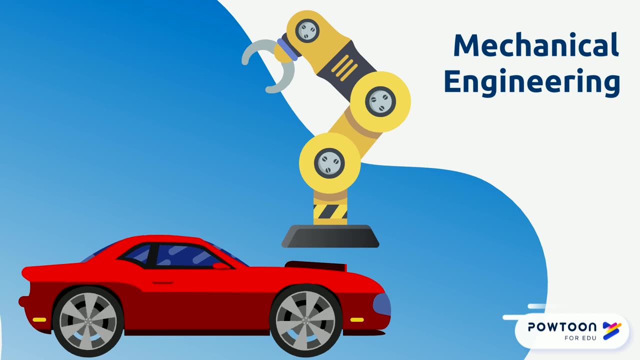 in our life, Things such as our cell phones and computers. Electrical engineers deal with creating electrical systems. It can be things as small as the device you're watching this on to entire power stations of electricity. Mechanical engineers create power generating systems. These are mechanical systems that involve lots of different machines and moving parts. 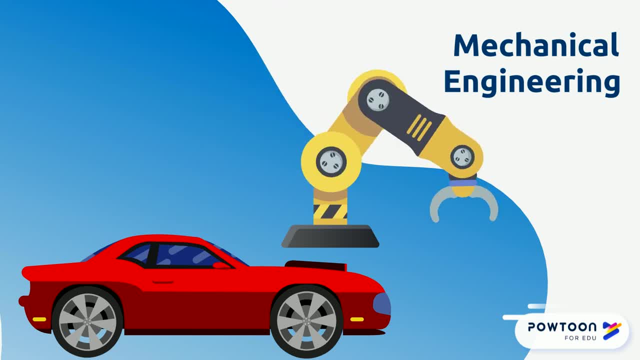 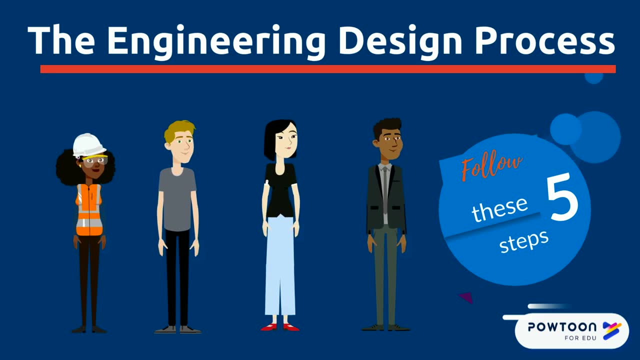 that make our lives easier. This includes things such as robotics, cars and elevators. Now that you know a little bit about different types of engineering, let's look at the engineering design process. This is the way that engineers get from their problem to a solution. 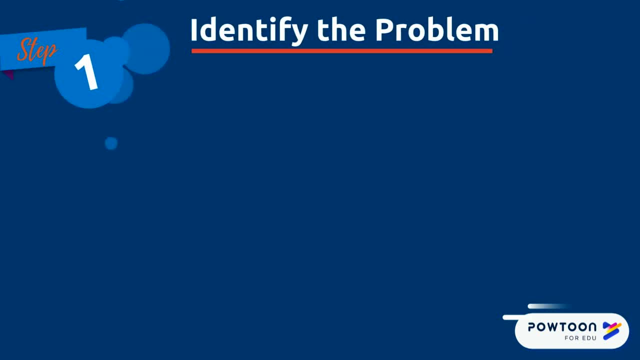 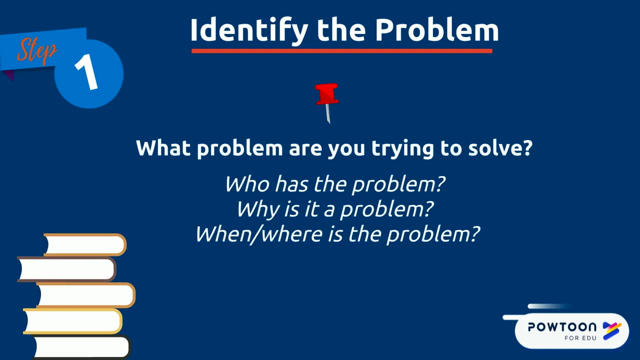 Step one of the engineering design process is identifying the problem that you're trying to solve. Not only do we want to know the problem, but we want to know more information about it, like who's experiencing the problem, why they're experiencing this problem. 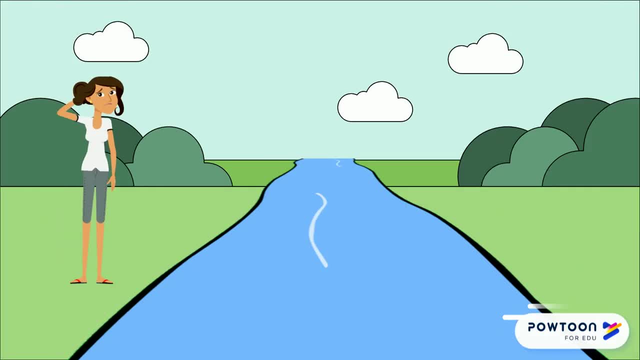 and where and when is this problem occurring? Let's take a look at an example. Our engineering friend, Maddie, is stuck on one side of the river. It would take hours for her to walk around to the other side of the river. How is she going to get across? 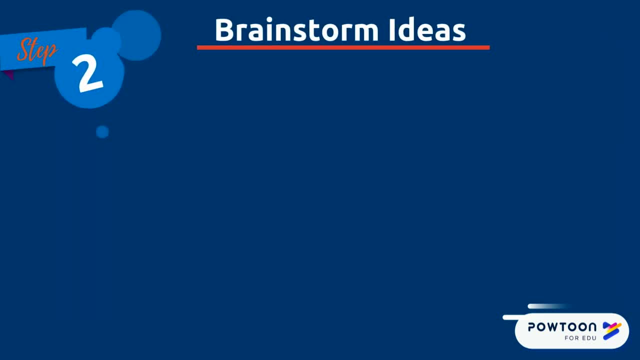 Step two of the engineering design process is brainstorming ideas. In this section, we want to think about as many ideas as possible and be open-minded to all solutions. In this stage, it's also very important to collaborate with our team members. We want to be open-minded to all solutions. In this stage, it's also very important to collaborate with our team members. 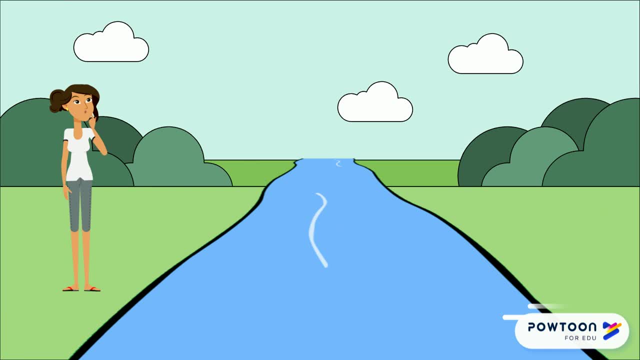 Let's get back to our example. Maddie is now on the brainstorming stage, so she's thinking about all the possible ideas. One example may be a boat or a bridge, or even a hot air balloon. There's no idea too crazy in the brainstorming stage. 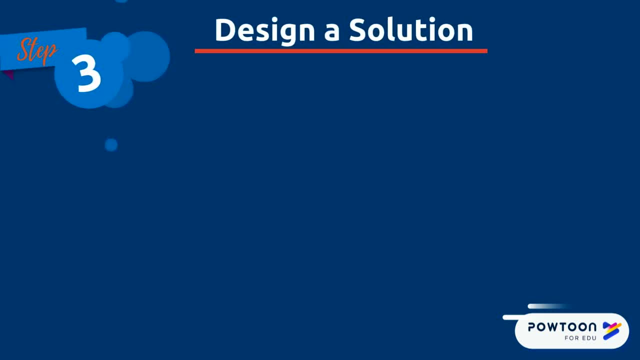 Step three is designing a solution. In this stage, you need to select one of your ideas or combine multiple from the brainstorming stage. but you need to be realistic. You need to think about materials. you'll need creating a design and even the cost and safety of the design, the materials you're using. 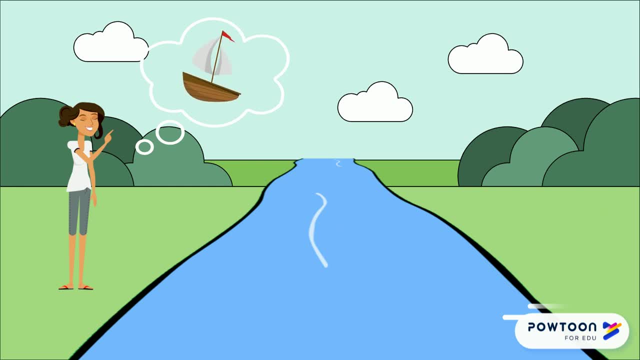 Maddie decides to go with the idea of the boat. During the design phase she'll have to think about the kind of materials and tools that she'll need. She'll have to get a paper and pen to draw out her design and a ruler to check her measurements. 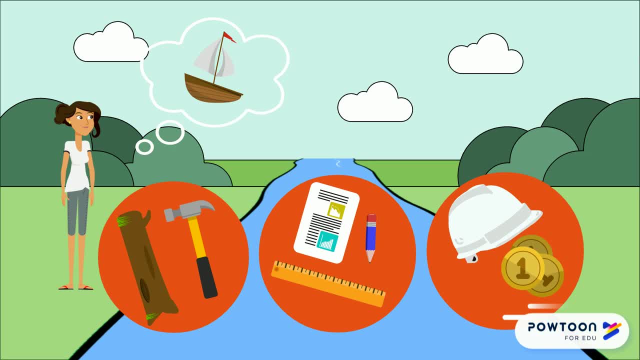 She'll also have to begin to think about safety and how she's going to get these materials when she goes to build. She'll also have to begin to think about safety and how she's going to get these materials when she goes to build. Step four of the engineering design process is make a model.